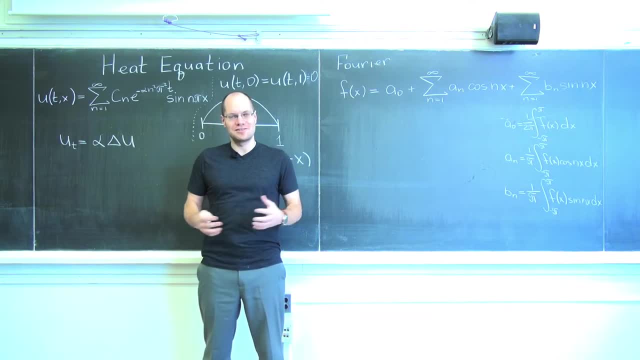 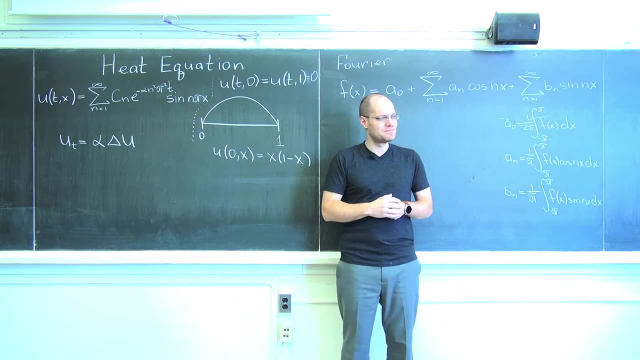 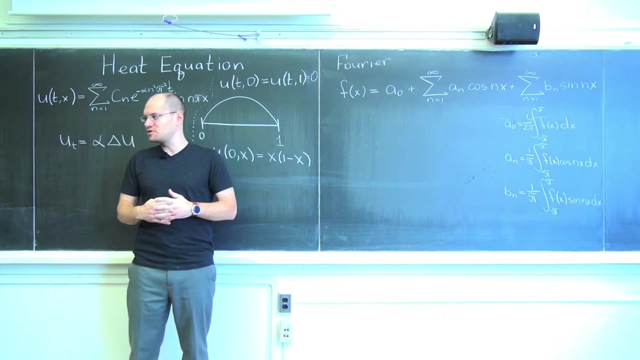 All right. so today we'll put it all together and we'll actually solve a couple PDEs on legitimate, albeit simple, domains. So over the last two lectures we did two things that were complementary and are now ready to be put together. 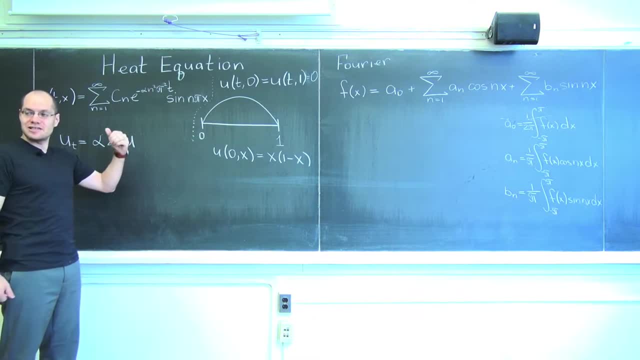 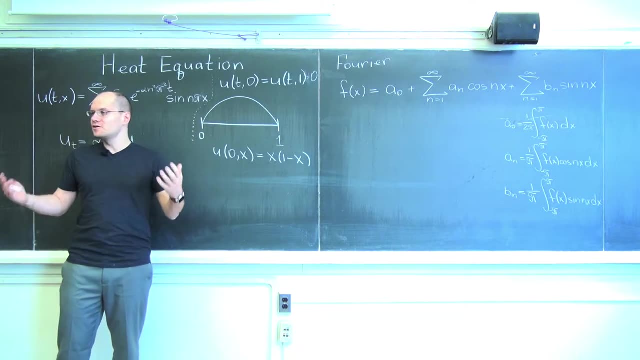 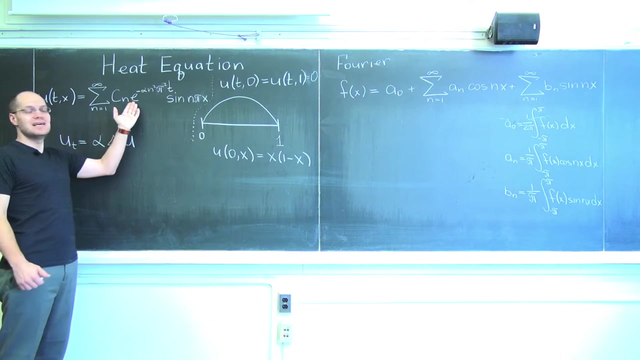 First we considered the heat equation and then the wave equation on a general domain and used separation of variables to show that the solution can be represented as a sum of terms, kind of like this: where there was an exponential decay in the case of a heat equation that multiplied some shape. 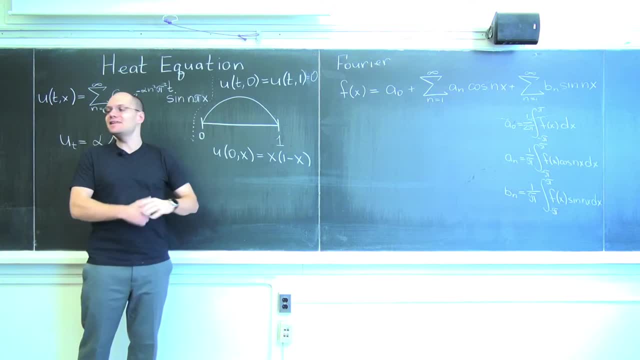 And that shape was determined by the domain and the boundary conditions. And so, then, we narrowed our attention down to the simplest possible domain, just a segment from zero to one, And then those shapes, I by the way- and by the way, by shape I mean just what the profile of the function looks like. 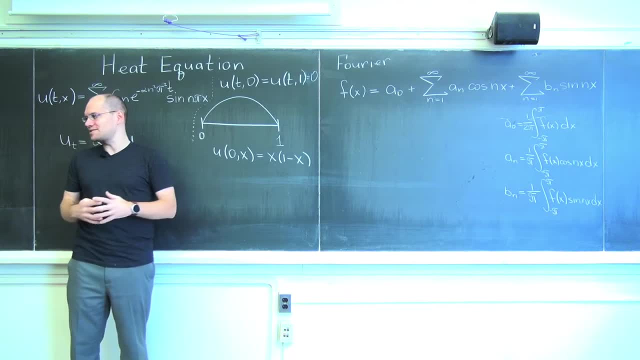 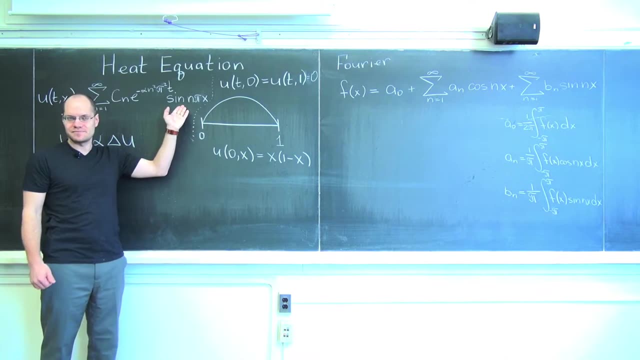 The eigenvectors, the eigenfunctions of the Laplace operator On the domain from zero to one. they just became signs, And not just any signs, specific signs, Signs with essentially an integer series. So I'll explain in a moment where pi came from and I'll reconcile some of the things that you see on the Fourier board. 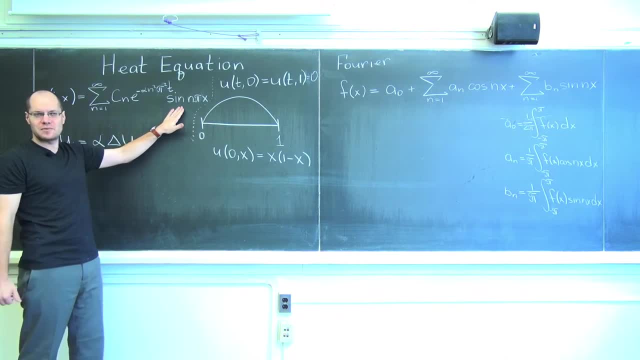 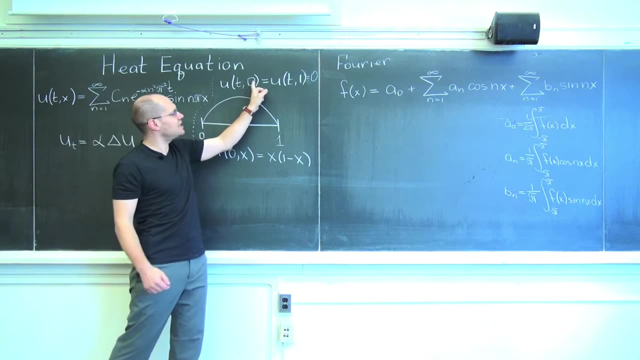 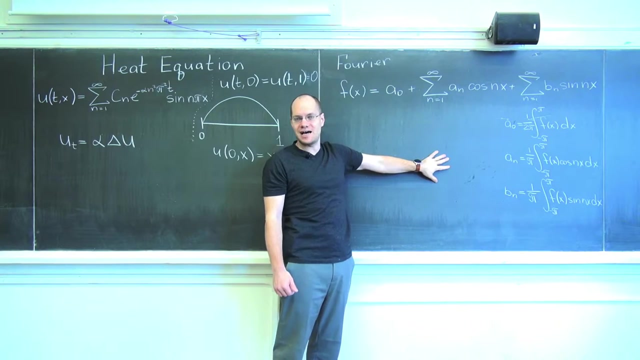 with this board, But that's the form that we obtained. There were also cosines that we threw out because they didn't satisfy our boundary condition of zero. So that should be a little bit suspicious, right? Because when in the last lecture, we talked about Fourier series, it was very clear that we needed both signs and cosines. 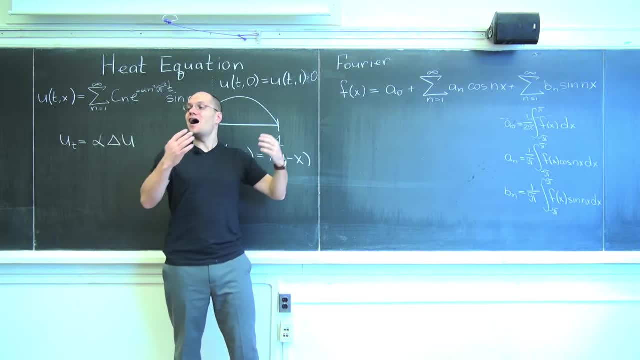 The signs took care of the odd part of the function And the cosines we needed to solve. We needed for the even part of the function, So we needed both signs and cosines. But this, excuse me, right here leaves us with signs alone. 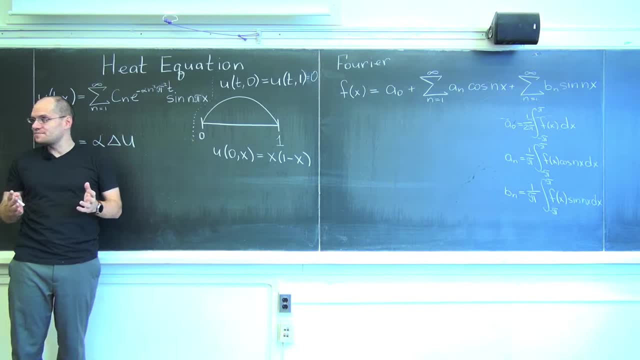 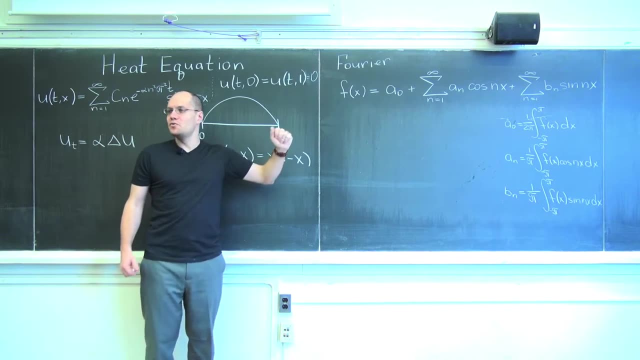 So maybe we don't have enough. Okay, so that's one thing we'll clarify. Another thing that's different is that when we were talking about Fourier series, we considered a segment from minus pi to pi. Let me kind of sketch it here. 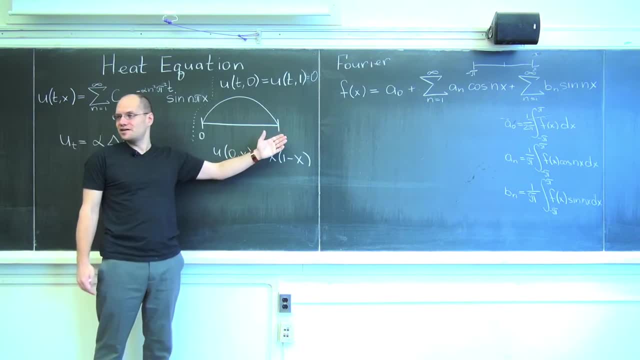 And here we're considering a segment from zero to one Or from zero to L, And you might say, well, that's not a big deal because it's just shifted and rescaled, So we'll just shift and rescale everything. Well, that's actually not going to be quite. 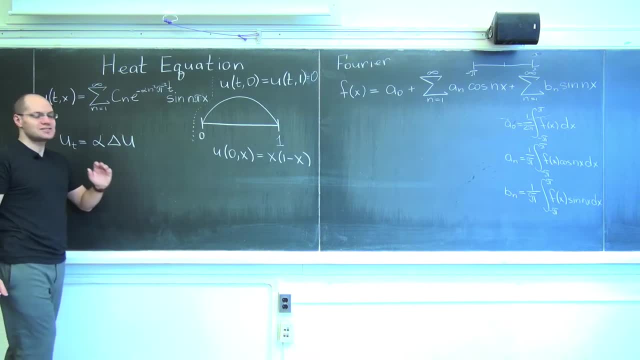 what we do. We'll do something a little bit different and I'll just convince you that it's enough. Yes, there will be a little bit of rescaling, But that's all there'll be. There won't be any shifting. Just to remind you. 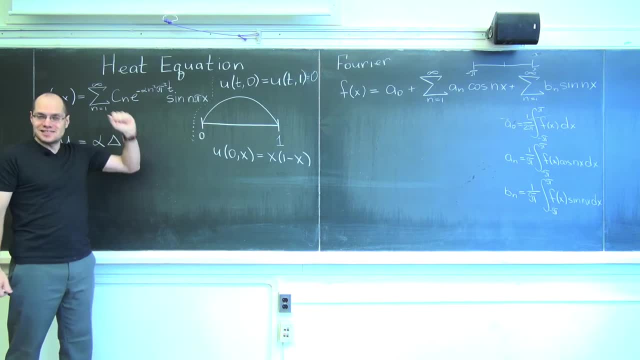 what the rest of the strategy was, Once we separated our variables and realized that in the case of the heat equation, it would be an exponential decay times, a corresponding sign where these ends are the same, and that's very important, And the signs once again. 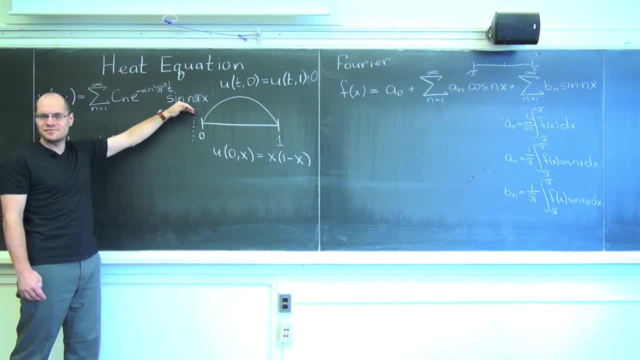 are the eigenvectors of the Laplace operator, with zero boundary conditions. The next step was to say: well, the equation is linear, so we can put them together into arbitrary linear combinations. And then calculus kicked in and we went from our conventional linear combinations. 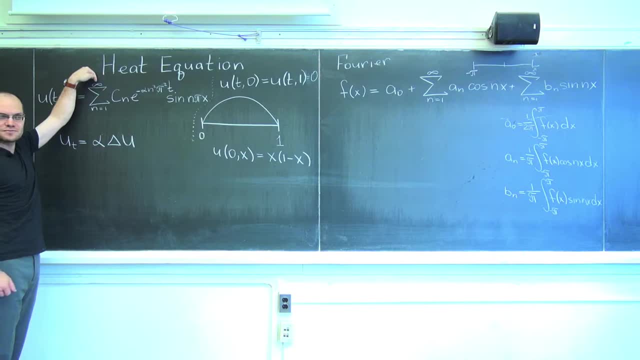 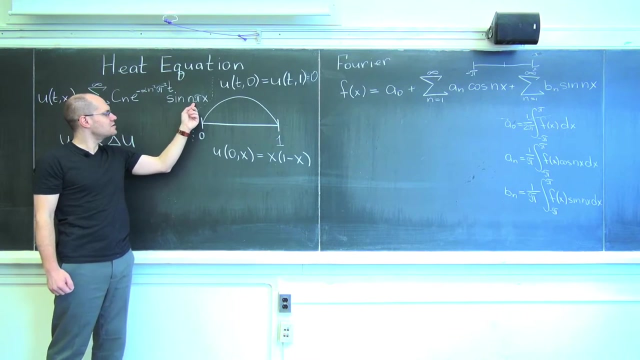 to linear combinations, so to speak, with an infinite number of terms, So in other words, infinite series. So this is calculus and linear algebra working together. And I will mention once again: I like thinking about the musical analogy, And it's this particular 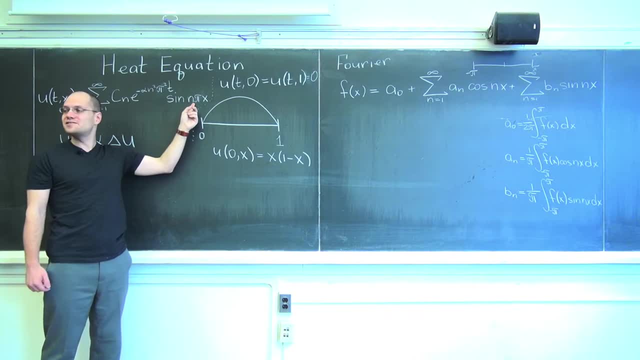 quantization, I think it's called, of the spectrum that makes stringed instruments, and actually all instruments, sound the way that they do. The fact that these eigenvalues, or these are the square roots of the eigenvalues, that the frequencies are proportional to natural numbers. 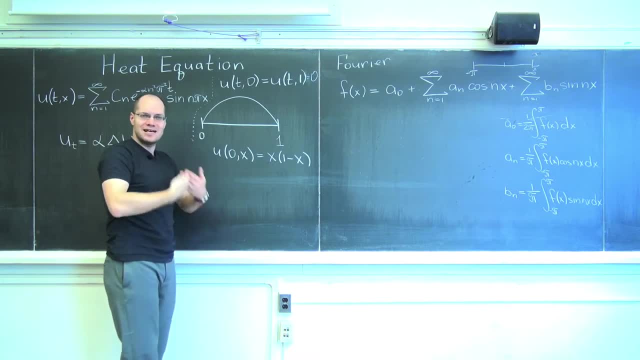 You get your base, one which is like this: when you pluck a guitar, maybe the most fundamental oscillation, and then you will see a string going like this. and then let me do it correctly like this: and those are the higher overtones, but they all belong to the same. 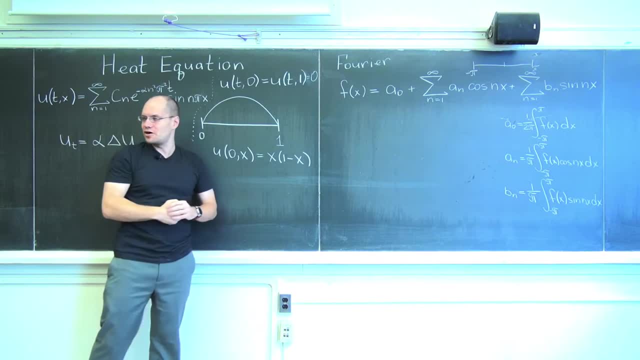 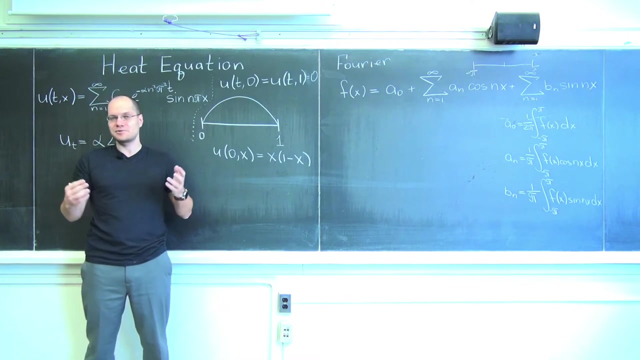 integer sequence, which will not be the same thing for the case of a drum, not even a square drum, We will see. we will find that the spectrum is quantized just like it is here, so there will be discrete values totally different, and that's why drums 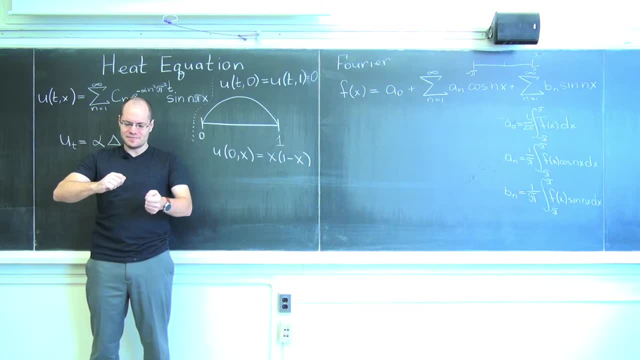 sound incoherent. and even what do you call the Caribbean instrument, steel drum. they sound a little bit incoherent. so your ear picks out the fundamental frequency of whatever indentation was hit. but then there is. it's a little noisy, isn't it? Well, that's because it's not a 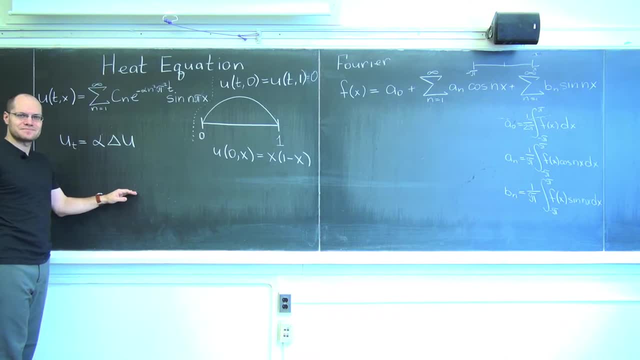 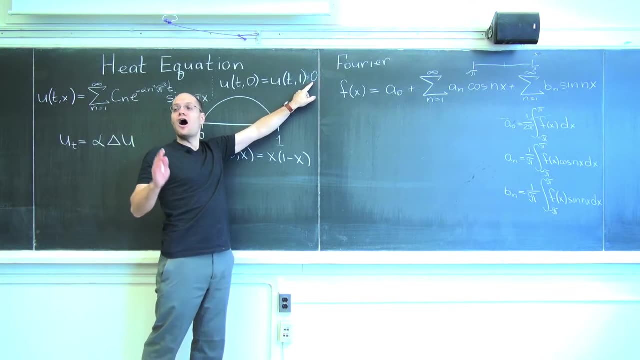 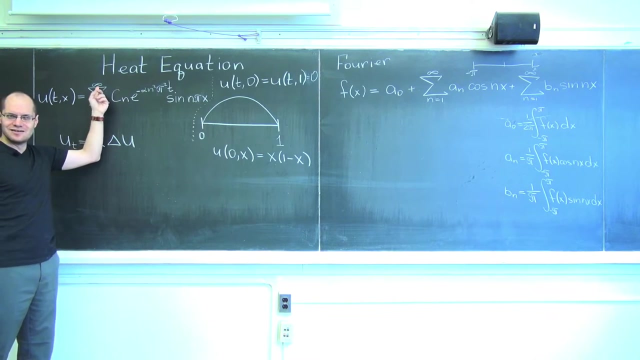 linear, one dimensional string. so that's something to keep in mind. So the next step in the strategy was to match the initial conditions. the boundary conditions being zero are kind of already taken care of by the sign. we have to be a little bit careful, because when you go to infinity, 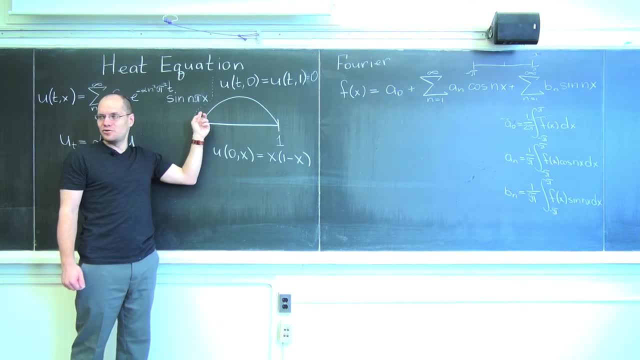 sometimes things can add up and they won't be zero in the limit. You have to be very careful about saying equals, whether it's the value of the function or its limit, from the left or from the right, okay, so you have to be a little bit careful. 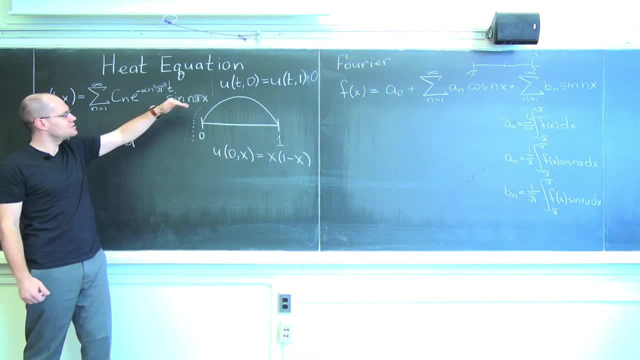 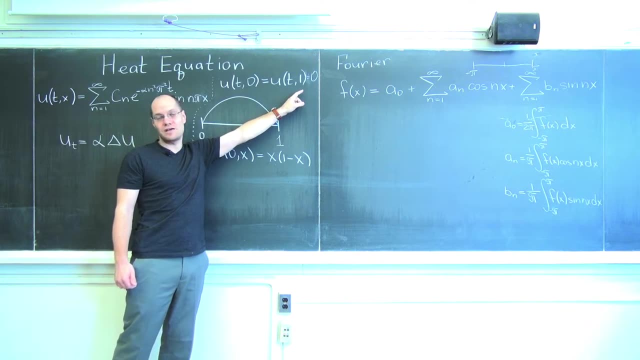 but let's just say let's save that topic for later. on an intuitive level, the fact that we're using sines and not cosines takes care of the zero boundary conditions. if they weren't zero boundary conditions, if this was the temperature in a room over a course of seven days. 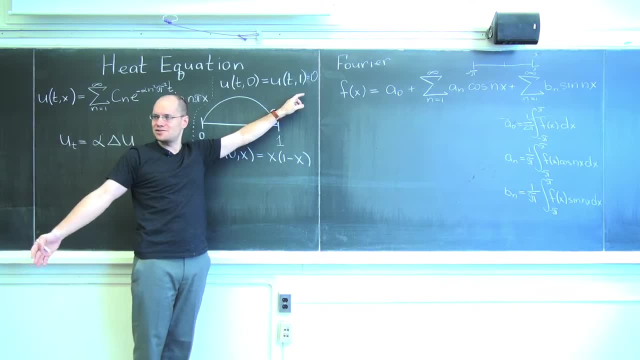 the sun comes up, the sun goes down. the sun comes up, the sun goes down. I would probably have some periodic and maybe not necessarily. maybe I would state the derivative of u and not u itself. these are called essential boundary conditions. these are essential boundary conditions. 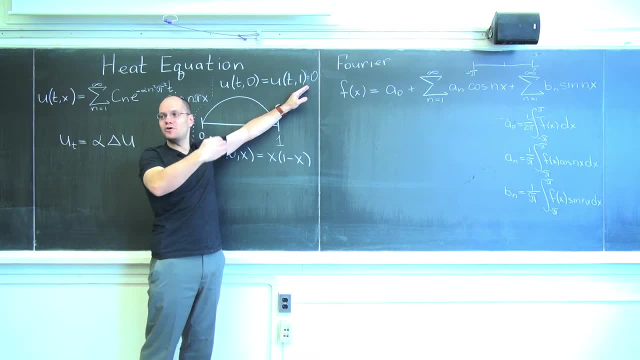 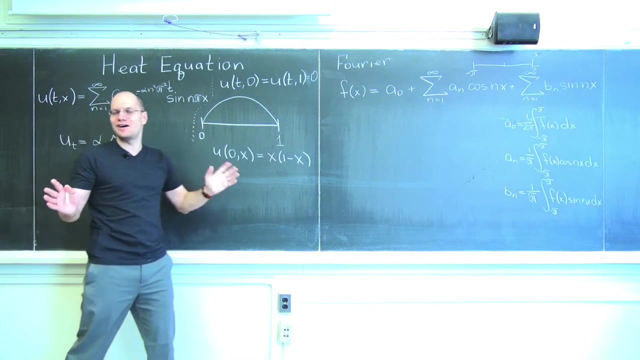 when you say what the temperature is and if you say what the flow of the heat is, then it's called essential boundary conditions, Neumann boundary conditions. so essential, natural versus essential and Dirichlet versus Neumann boundary conditions. in any case, terminology. we'll talk a little bit more about it when we get there. 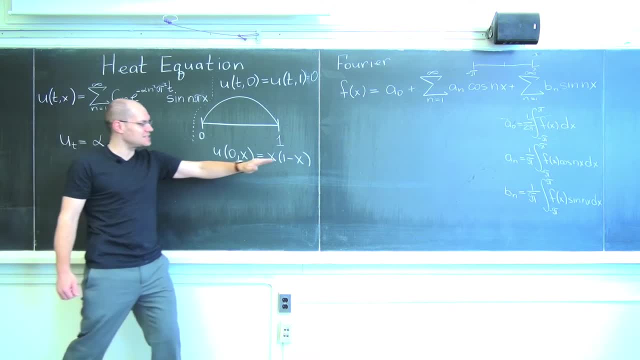 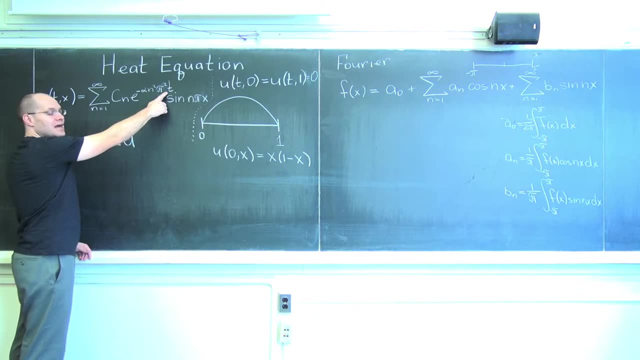 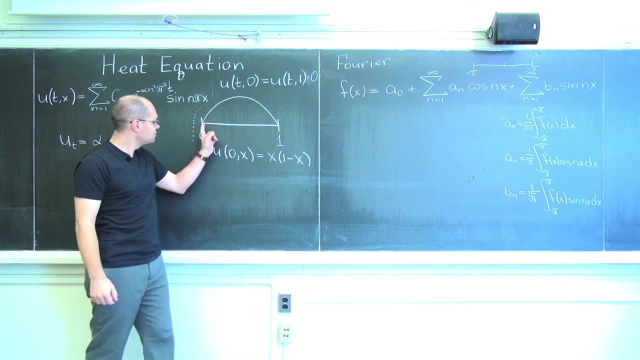 okay, so the name of the game was satisfying the initial condition. and what did we do there? we plugged in t equals zero and we were left with this series that had to match this initial condition, and I chose initial condition carefully so that the values of the boundaries 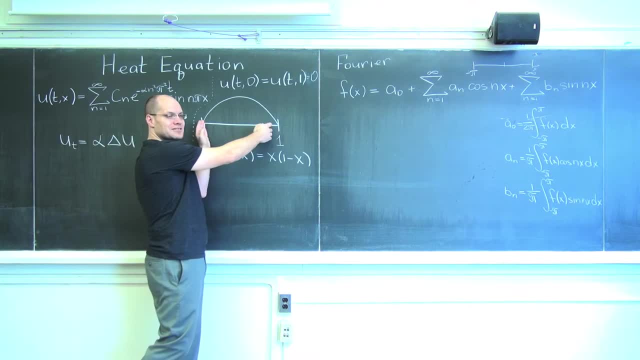 are zero, so we don't have a mismatch between boundary conditions and initial conditions of the corners. so that's fine. there could be a mismatch too. those are very interesting problems as well. we just don't have them with us. so we plugged in: t equals zero, and what we realized? 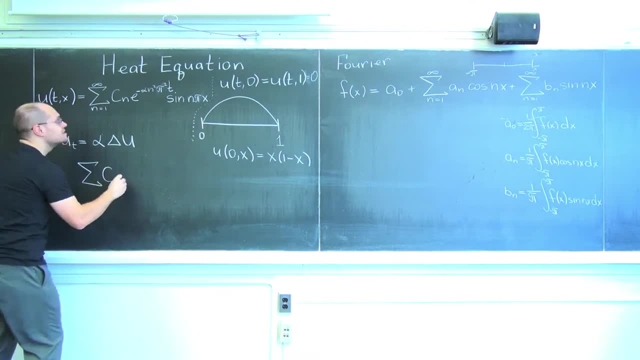 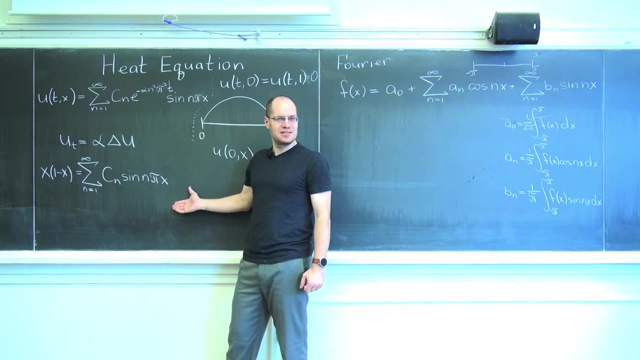 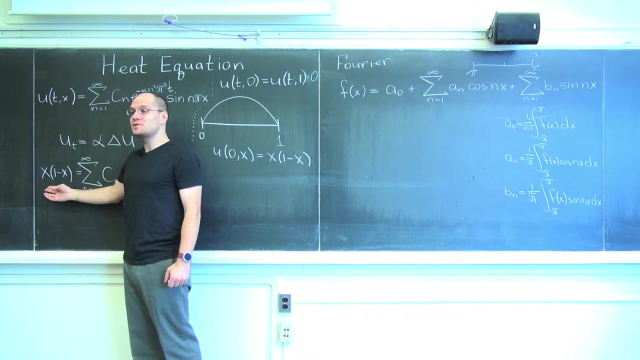 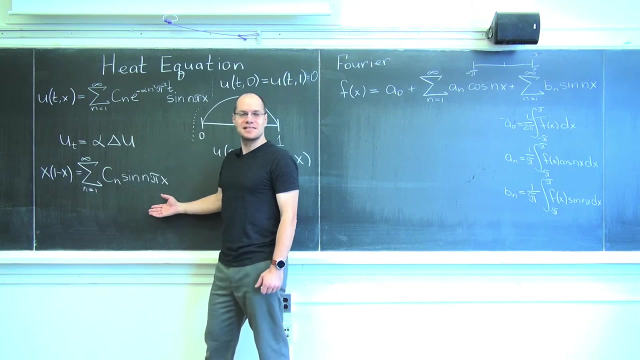 is that we have this series. so when we plugged in zero we got what looks like half of a Fourier series and it must match our initial condition. so at that point we said we're faced with the problem of decomposing any given function as a sum of sines. 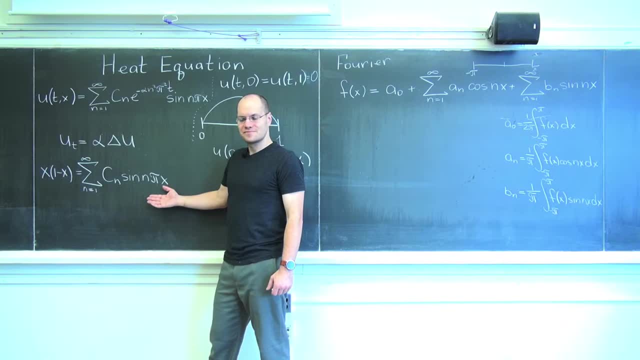 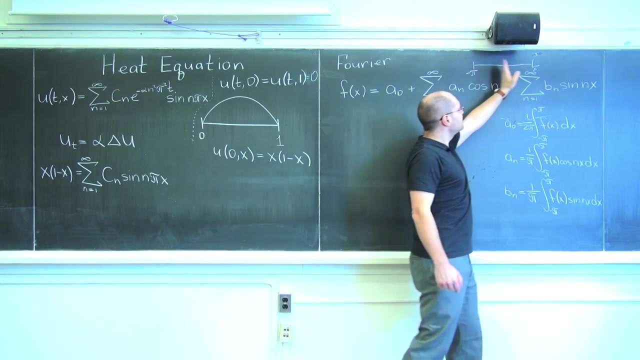 and no cosines. so we left ourselves with this problem. and then in the last lecture we kind of addressed this problem, but in a different way, slightly different way. so we'll now reconcile the two somewhat carefully. we looked at a sigma from minus pi to pi and took a function that was periodic. 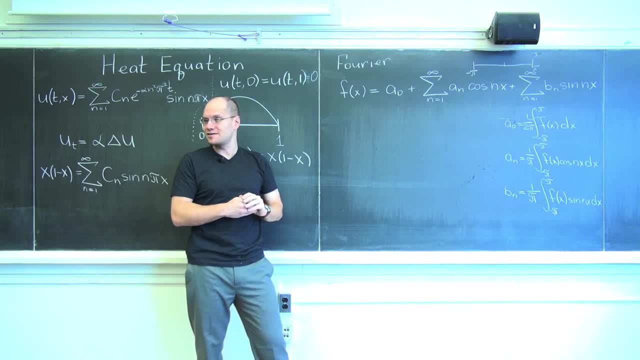 from minus pi to pi, not necessarily zero at the ends, but just periodic. and that requirement made even the simplest functions- for example f of x equals x in the periodic continuation sense- became discontinuous. that was fine. and then we decomposed it as a linear combination of sines and cosines. 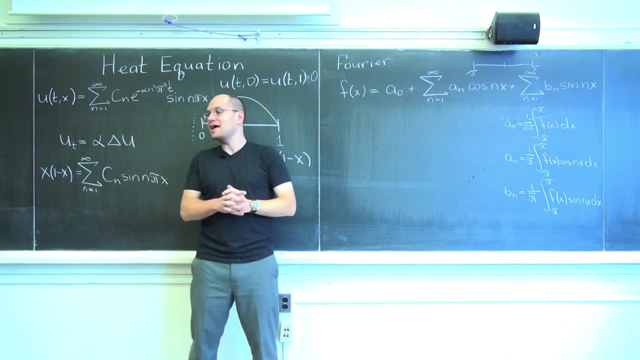 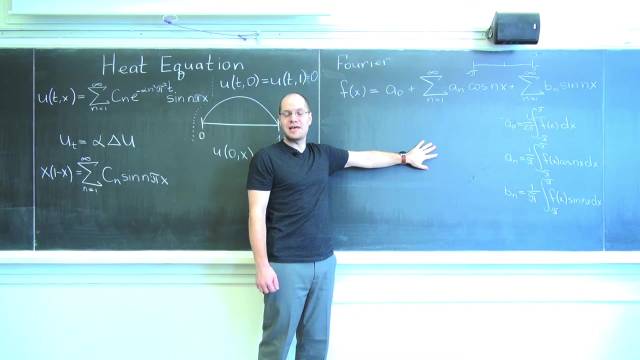 and we kind of concluded that it's possible for just about any reasonable function if you define very carefully what it means for an infinite series to equal a function. so our conclusion from the last lecture was that any periodic function can be composed as an infinite Fourier series. 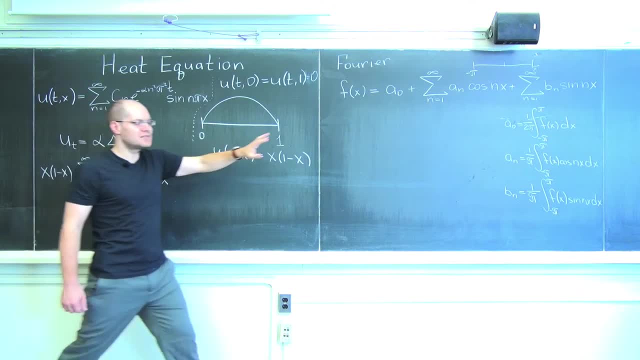 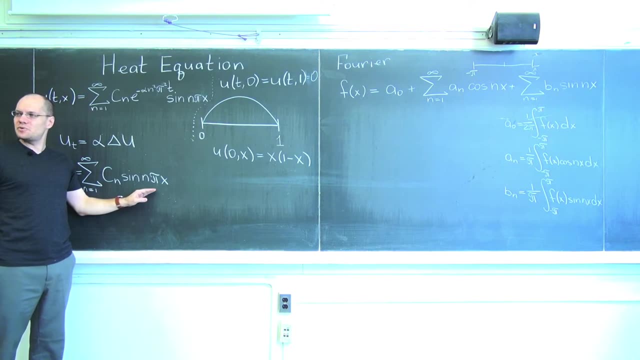 and that was great. now we have to reconcile the two. how does this finding help us here, where we're left only with sines? it seems like we have half the functions- that's number one- and that the machinery would have to be reinvented for this case. 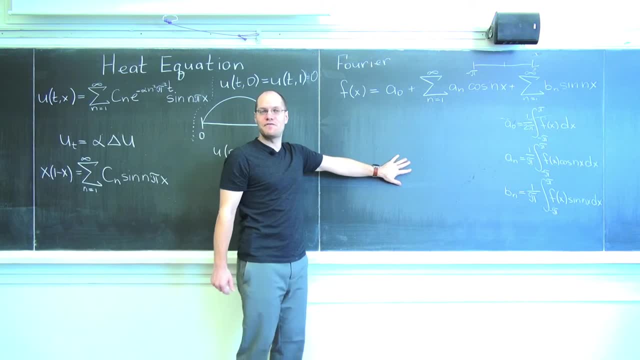 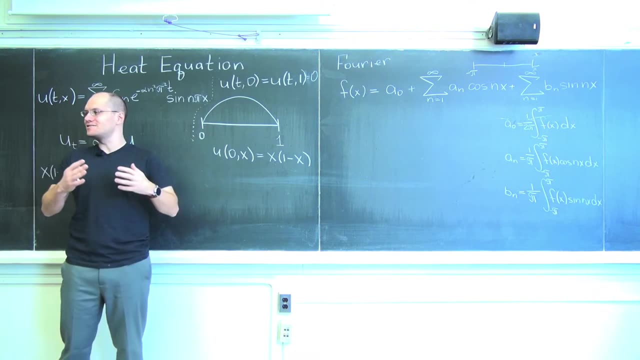 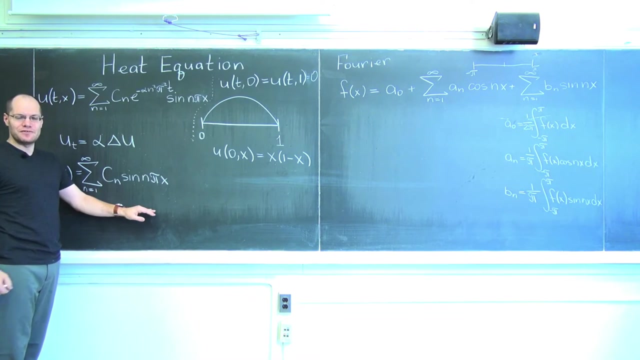 well, we can actually reconcile this and with Fourier series, and here's why it should work on a simple count basis. yes, in either case there's infinitely many functions, but I just want to convince you that it's kind of the same number of infinite functions, because here we considered 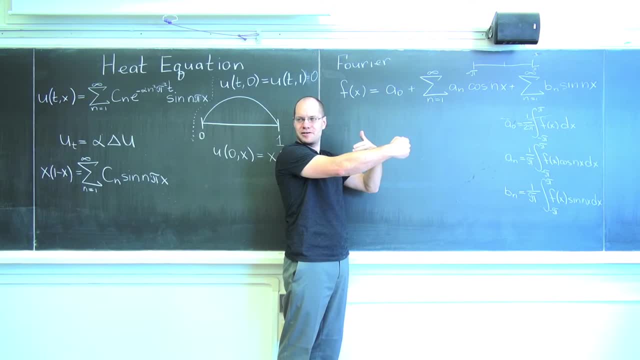 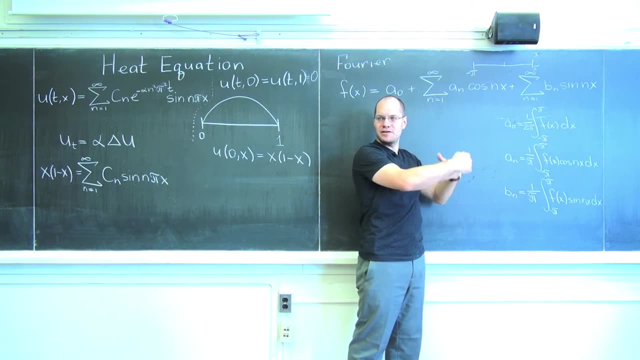 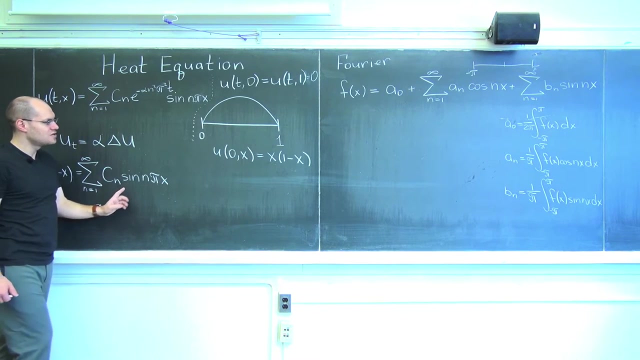 sines and cosines. that started with having a single period that was the lowest, let's say, cosine, and then half the period, one third the period, right, in other words, that base frequency, twice the frequency, three times the frequency, four times the frequency, and so forth. but here 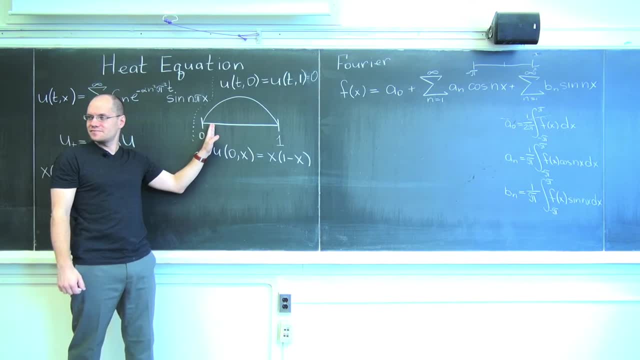 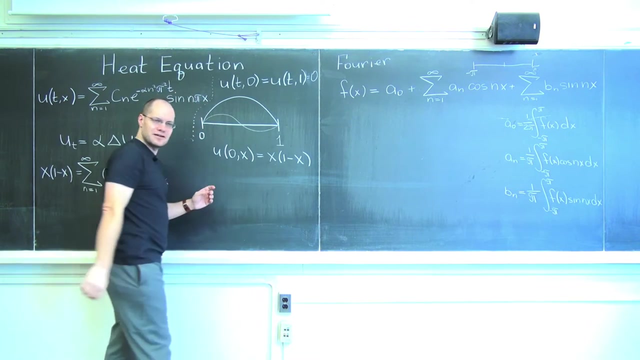 if you look at this series relative to this segment, we're allowing ourselves the sines of half the frequency right. if we were solving the same Fourier series problem as we did last time, this one right, that would be the lowest frequency sine that we would allow ourselves. 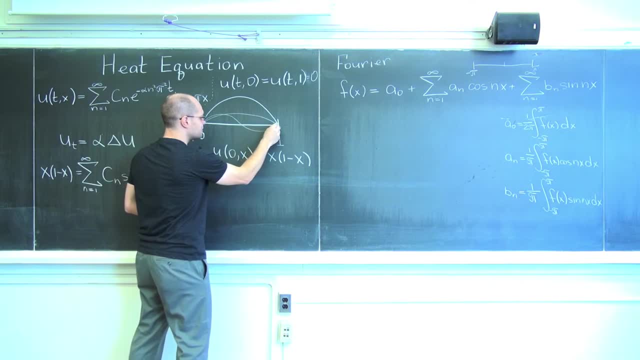 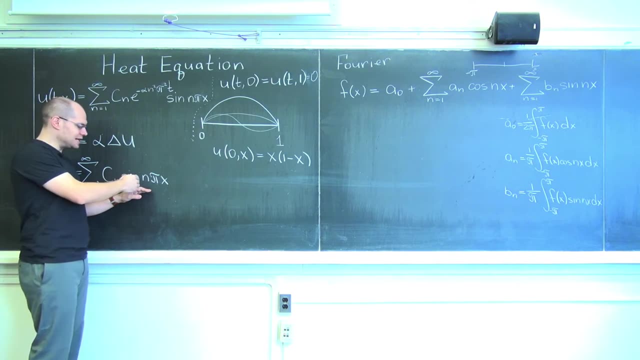 but here we're allowing ourselves this sine. so half half the frequency. so yes, it's half the functions, but because we're allowing ourselves half the frequency, and then there will be one with three- let's call them half wiggles, it will be three halves frequency. 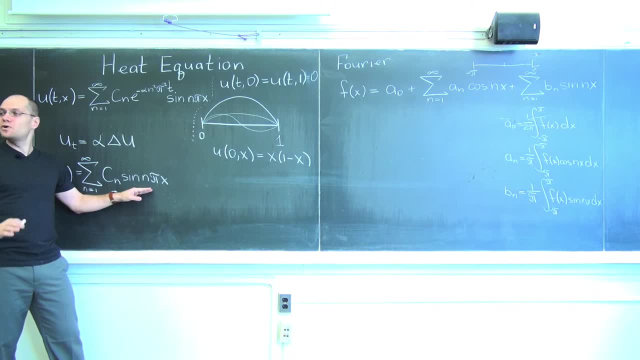 so it's actually the same number of functions. so we're okay. so it's not like we have half the functions. we have the same number of functions and these functions are nice. I keep repeating it. I keep repeating it because it's the statement that generalizes. 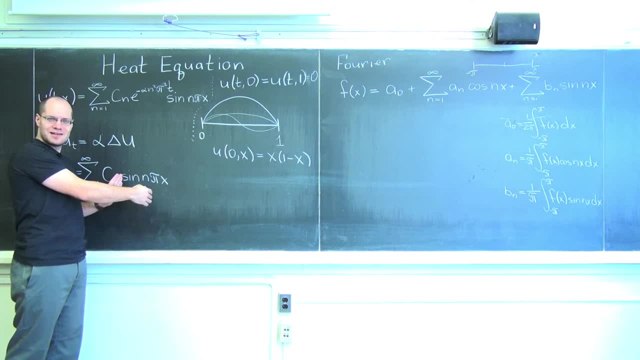 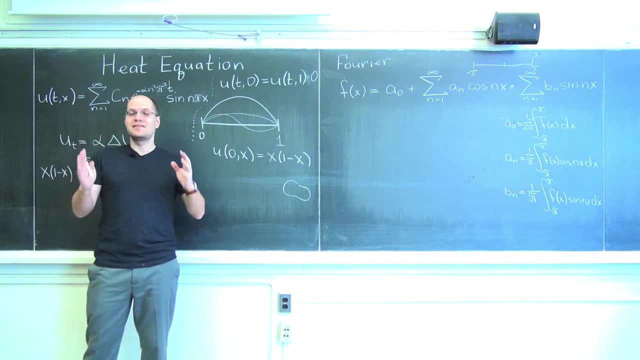 there are several reasons why we want to stick to these functions. it's not just because they match the boundary conditions, but because it's these functions that are the spectrum of the Laplace operator with zero boundary conditions. okay, so now let's think through the practical question. 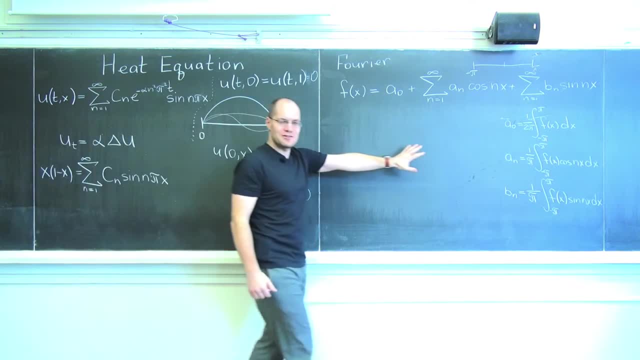 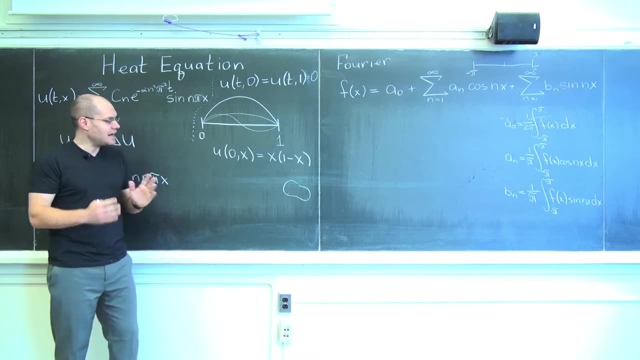 of using these formulas without or analogous formulas, without having to re-derive them from scratch, and it works very simply. so I think you understand where the multiple of pi comes from. the multiple of pi comes from the shrinking of this segment from zero to pi to going to zero to one. 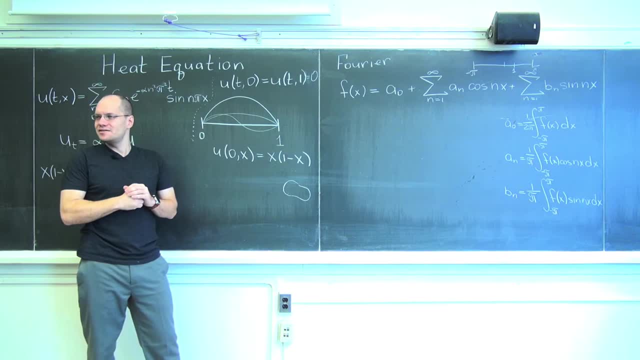 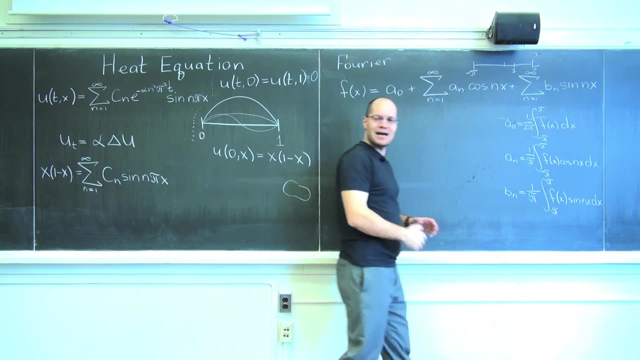 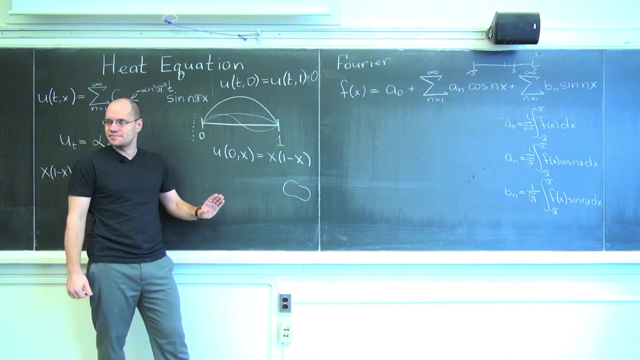 so that's easy to imagine, although we'll think very hard about what happens to this scaling factor. I haven't thought about it. I didn't think about it before the lecture, so we'll think about it together. there will need to be an adjustment there. okay, but what are we going to do about? 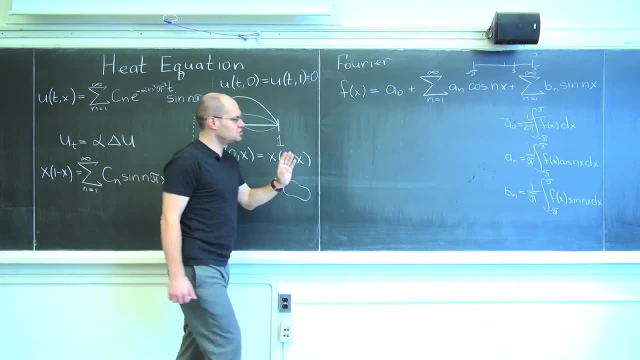 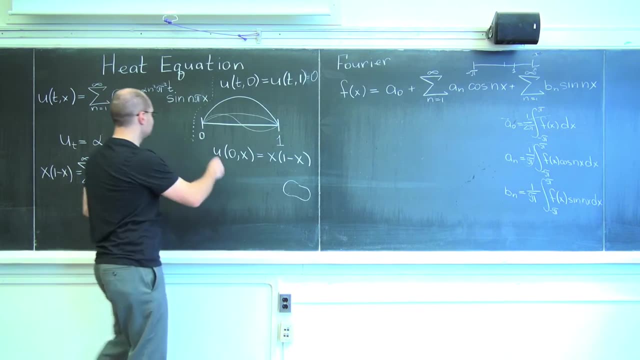 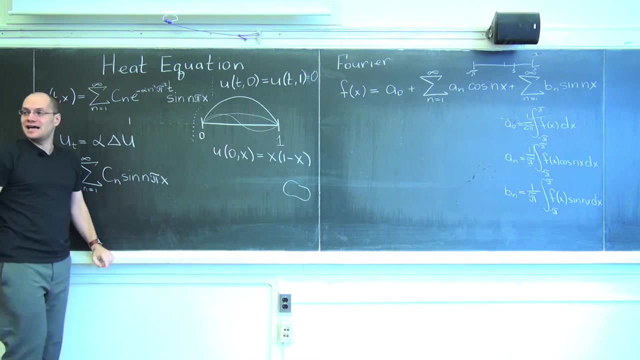 the left side. here's what we're going to do just to make this scenario. in the case of this scenario, we'll imagine artificially that we're actually doing it on the segment from pretty good minus one to one. so we're going from minus one to one. 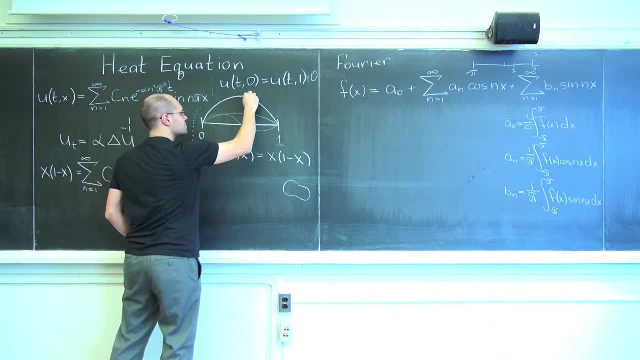 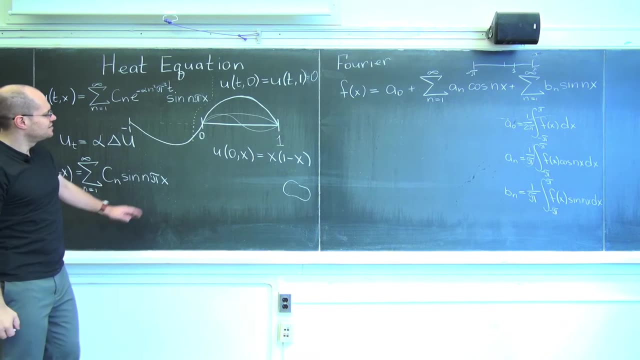 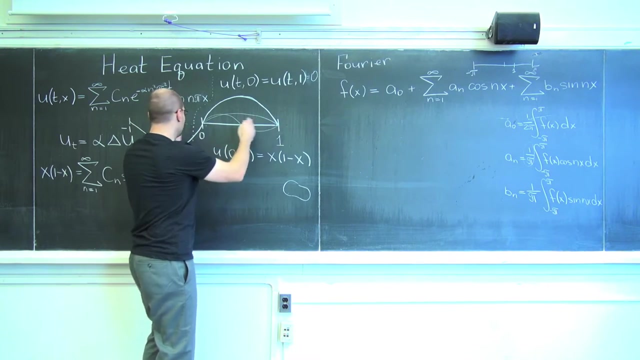 and we're going to continue our initial condition in the anti-symmetric way like this. see what I did. so now, instead of taking just this part and representing it in terms of sine with half frequencies, we will kind of: is it good enough? it's hard for me to let it go. 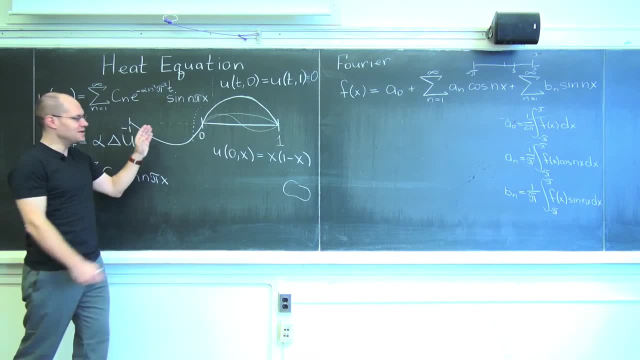 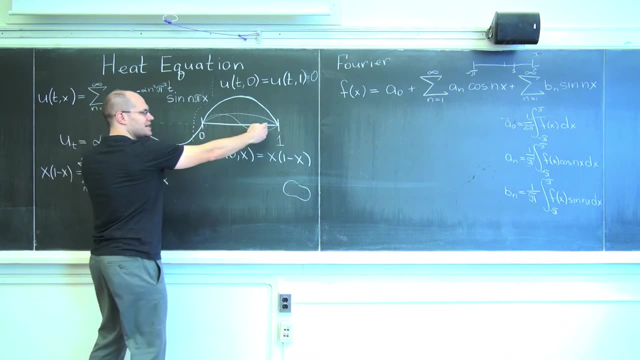 but I'll let it go, we'll just pretend it's perfect. we'll now use this larger function, this anti-symmetric odd function on the segment from minus one to one, and we'll think of this function as being fit to a legitimate Fourier series with sines and cosines. 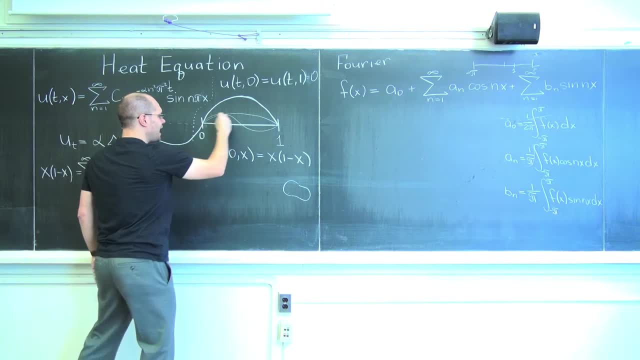 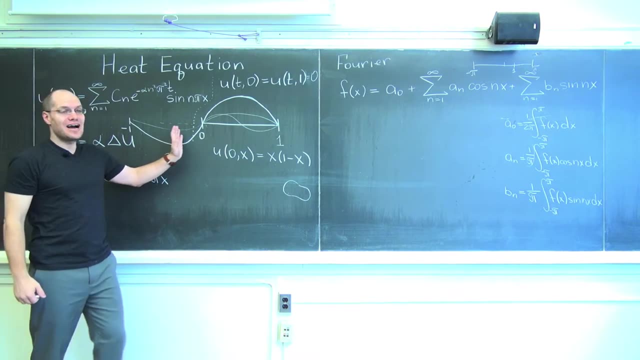 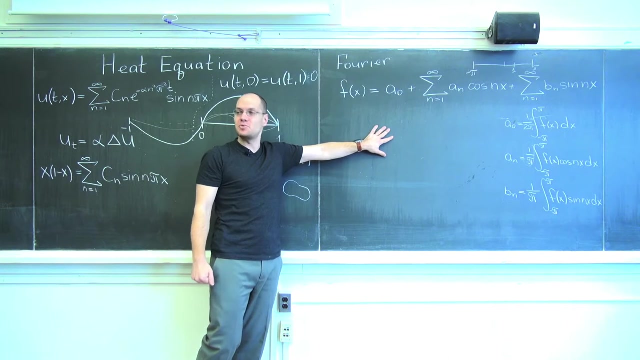 on this double period. so whatever was a half wiggle is now a full wiggle- same problem. so we're now back in this scenario. it's just that from going, instead of going, from minus pi to pi, we're going from zero, from minus one to one. 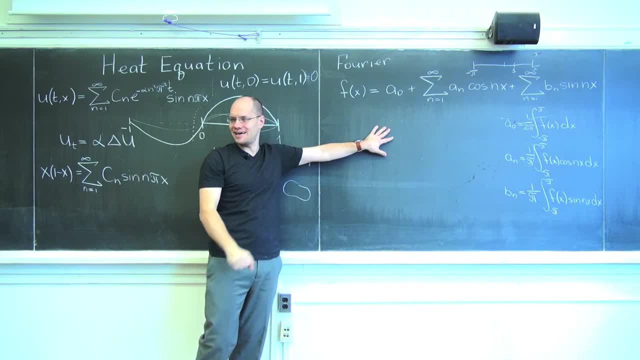 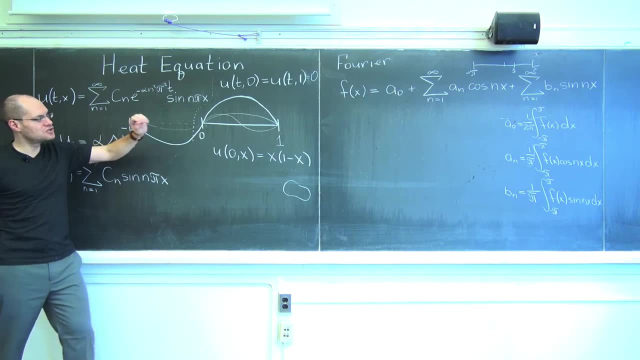 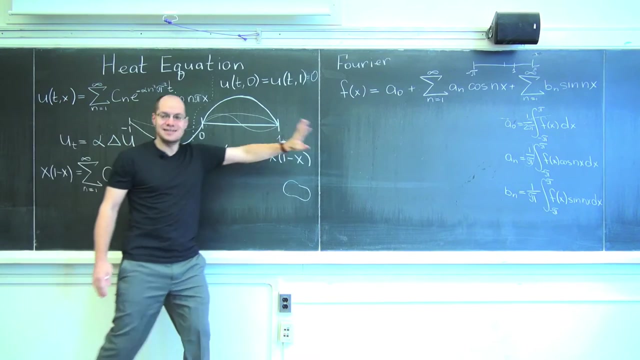 so we just have to put the right scales of pi in the right place. and because this is an odd function, there is no a zero, there is no a sub n, in other words, there are no cosines. so it's nice how what we did in last lecture now fits. 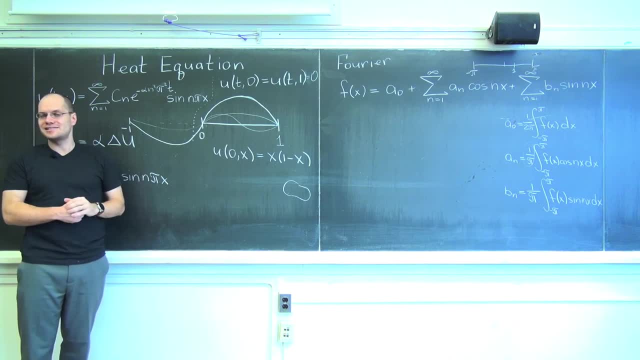 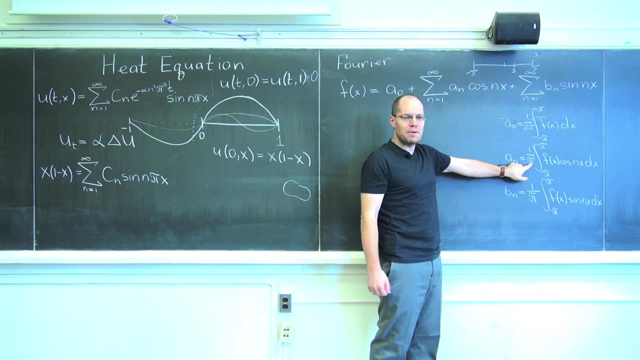 so there are no cosines, so there are only sines, so there are only a sub n's, which we're calling here c sub n's, and let's just write down what c sub n is very carefully, because remember where this one over pi came from. 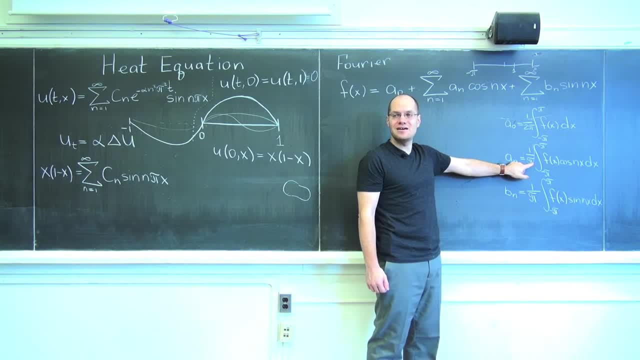 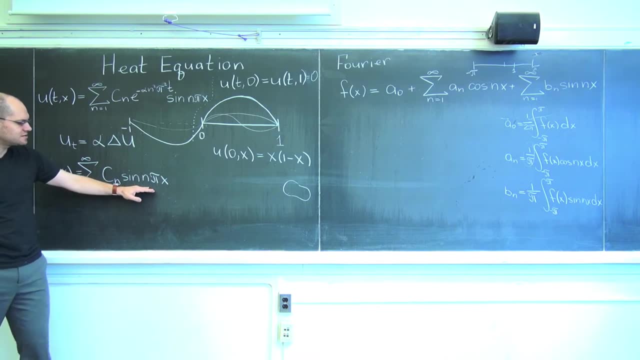 this was the integral of sine itself. okay, but now our functions are not sines and cosines, because we're going from minus one to one. they're now sine n pi x and cosine n pi x. that's where this scale goes. so for sure we will have this c sub n. 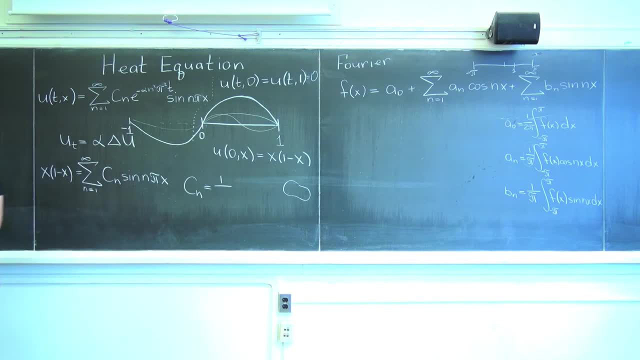 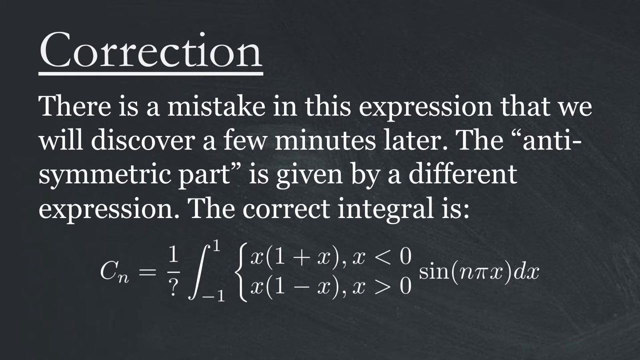 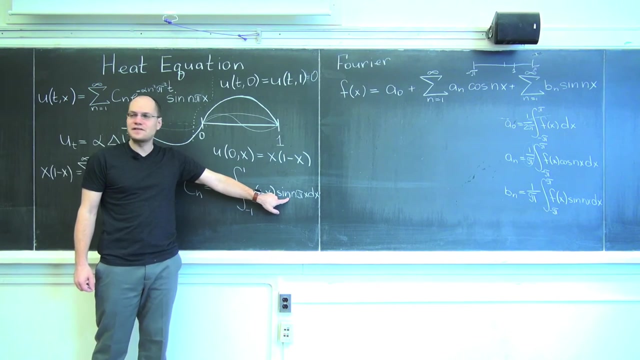 will be one over something. we're about to discover what it is okay. and this thing right here is the integral of this function squared, and let me think about it as a I don't know on an intuitive level. we're not going to do a proper integral. 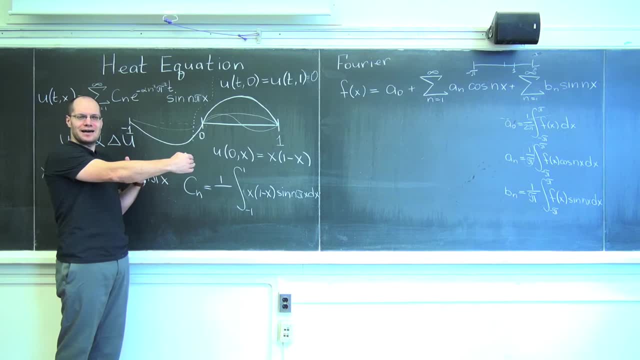 when it was stretched from minus pi to pi, that integral was pi. but now we're shrinking it by a factor of pi, so the whole picture gets shrunk by a factor of pi, so the area gets smaller by a factor of pi. so I think it's one. 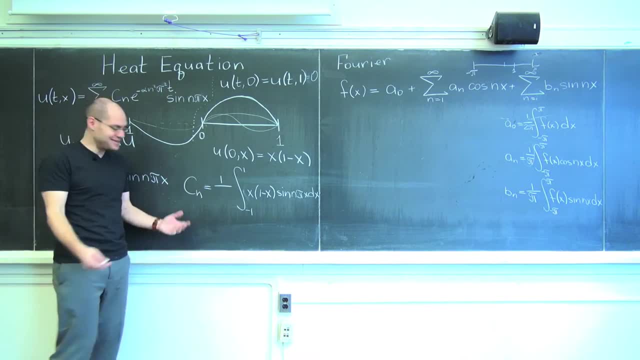 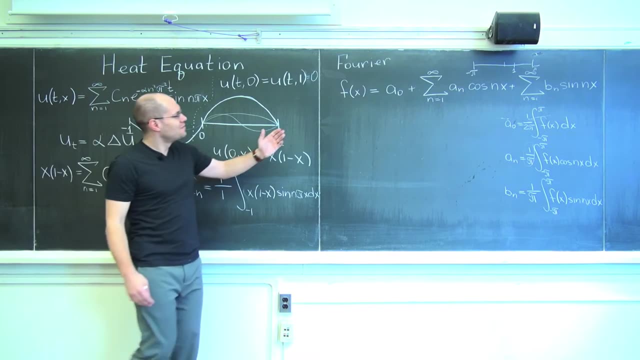 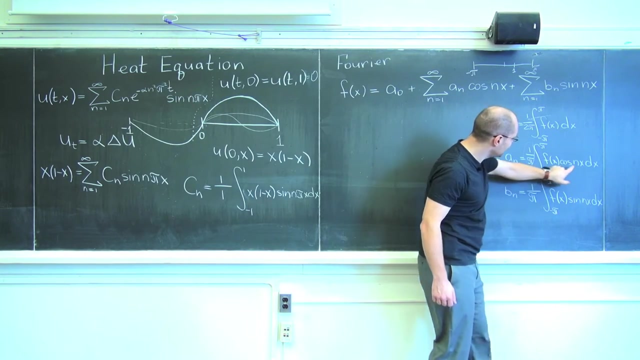 is that why you were going like this? okay one, that's not what I expected, very nice. so maybe going from minus pi to pi actually would yield a slightly cleaner, Fourier series. it would move these pis into the sines and cosines and then a simple change of variable. 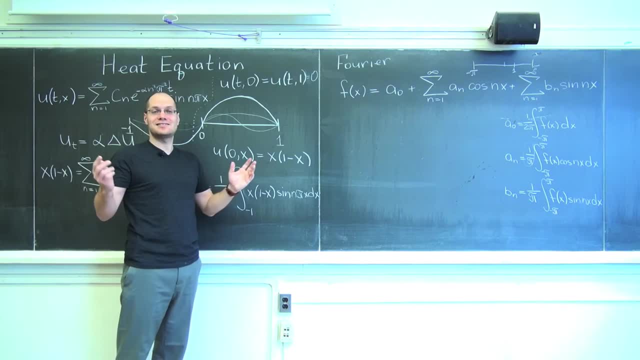 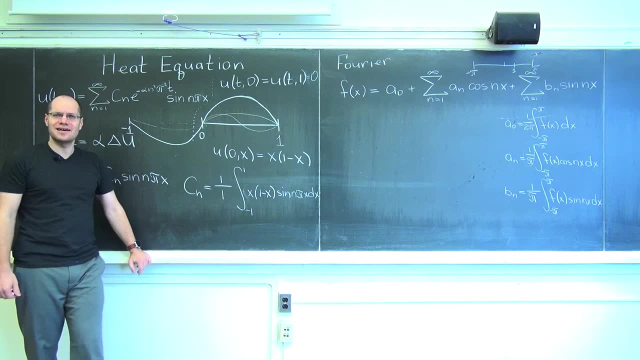 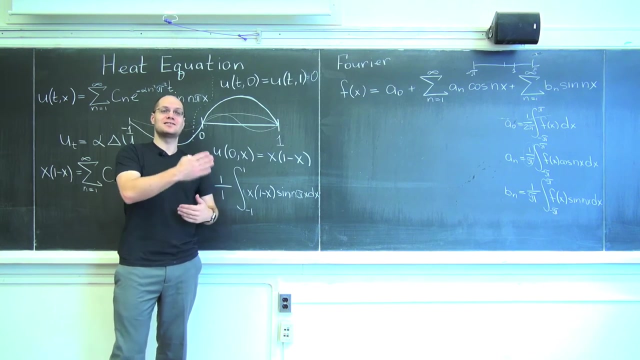 shows you the equivalent: fantastic, fantastic. so if we had considered that, surely we would have discovered that, yes, perfect, yeah, no, of course it is, it's just a rescaling. but the only problem with the rescaling that you have to solve is whether it's one over pi or one times pi. 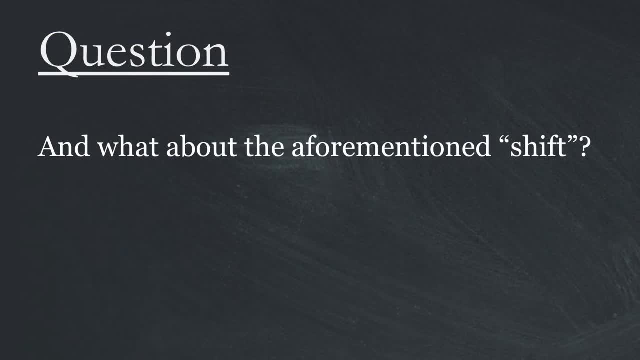 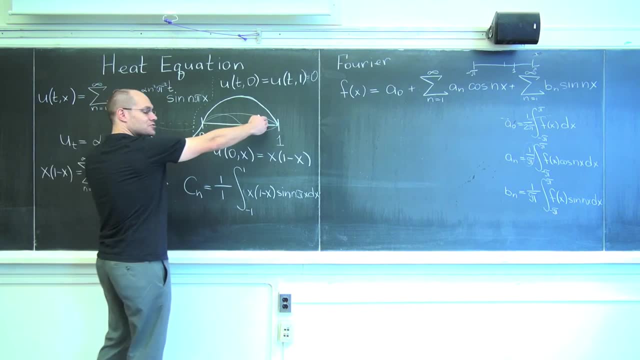 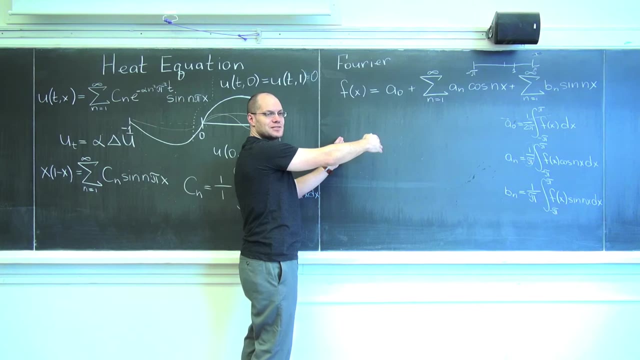 you just have to put it in the right place. no see, we don't have to do a shift because we did the symmetric flip. everything's in the right place right now. we made this new picture a special case, if you allow for rescaling of the old picture. 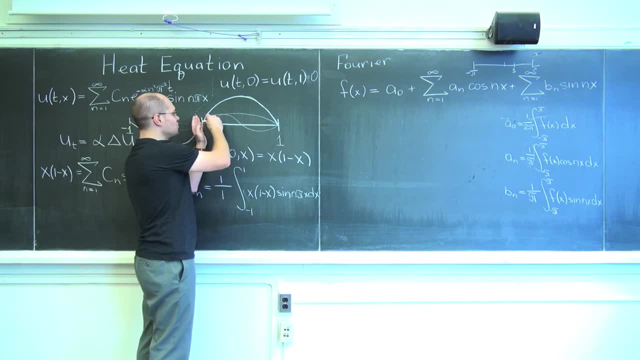 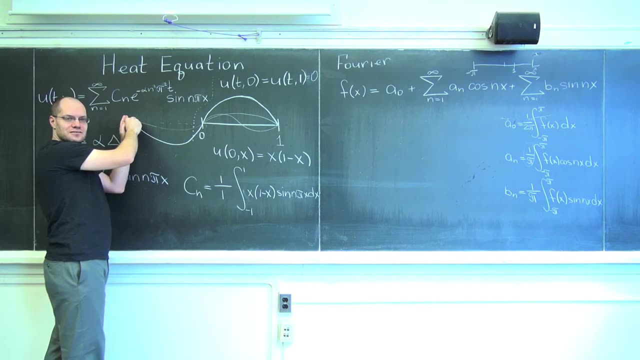 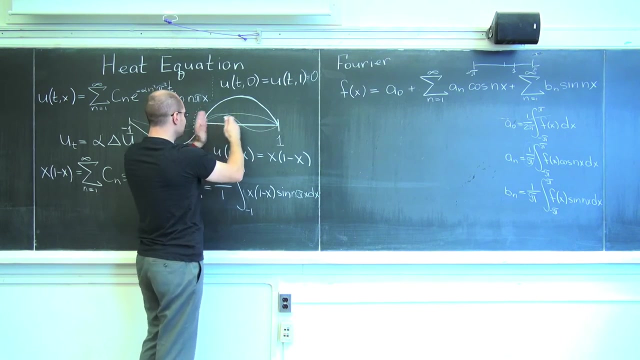 so there's no shifting anymore. here's what we did. we said, instead of doing this part, let's do this larger function, and then this would be just the part of the overall thing. that's right. so we're kind of doing it here, but we're ignoring this part. 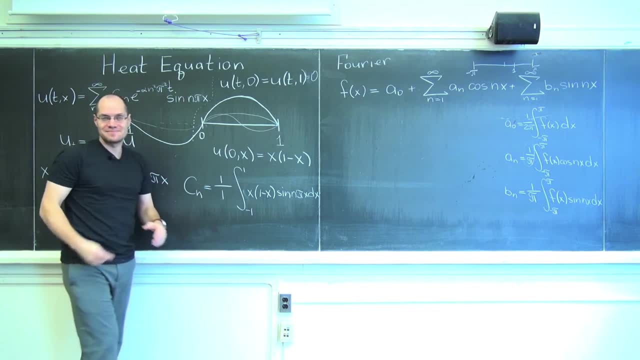 we only added this part to make this a special case of that. ok, so all we're left with is having to evaluate this integral, our integration genie. I was about to call you an integration fairy, and then I thought that would not be right, so the genie will tell us what this integral is. 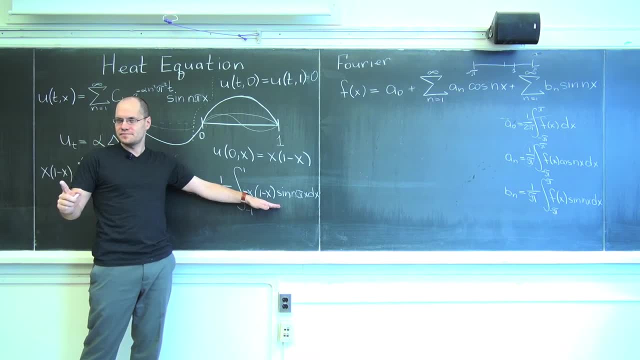 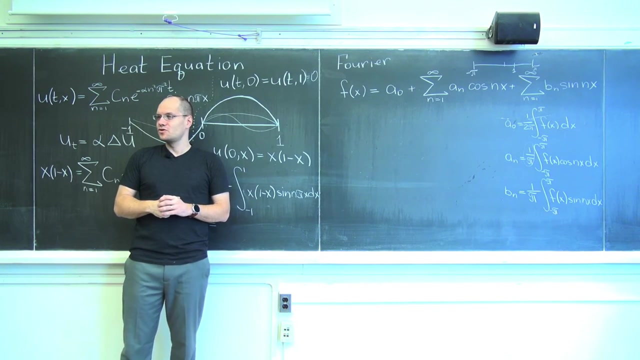 accounting for the fact that n is an integer, so he won't say cosine n, pi or anything like that. he'll just tell me the answer, and it's Wolfram. Alpha deserves the credit here. well, while he's doing that, let me ask you a question: how fast do you think? 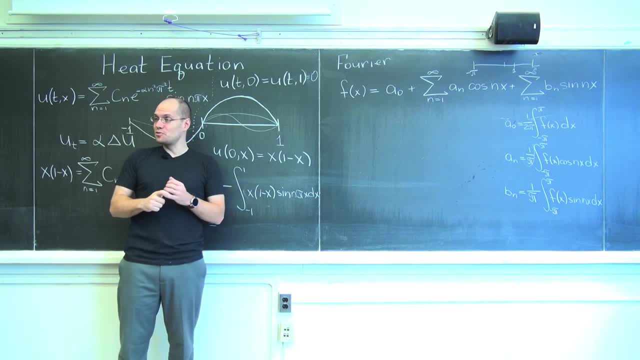 the coefficients will be decaying. that's a great question because, remember, if it's continuous, they go down as one over n, they decay as one over n. if it's continuous but it's derivative is discontinuous, then one over n, squared. if it's derivative is continuous. 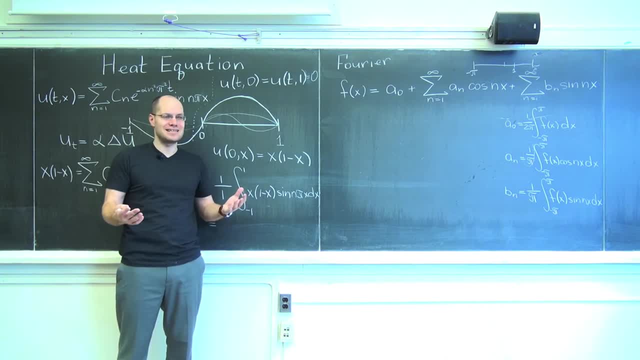 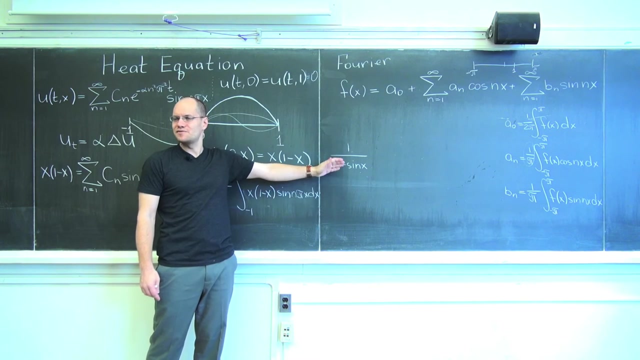 one over n to the third, and if it's perfectly continuous in the periodic repetition sense, can you even think of a function like that? I'll show you one that's perfectly periodic. it actually takes a moment to think of something like this, because if you, that's both. 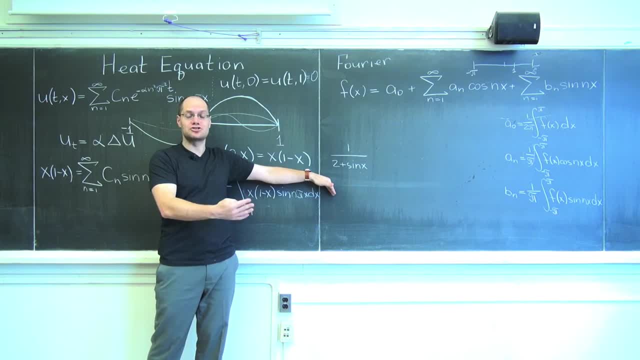 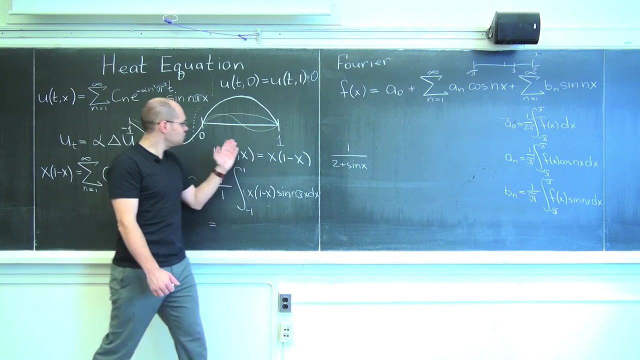 infinitely periodic, infinitely continuous, but also not trivial, like a finite sum of sines and cosines. so that's a good example. so the coefficients for this function from minus pi to pi, would be decaying exponentially. so what do you think the case here is? and remember, we're doing this function. 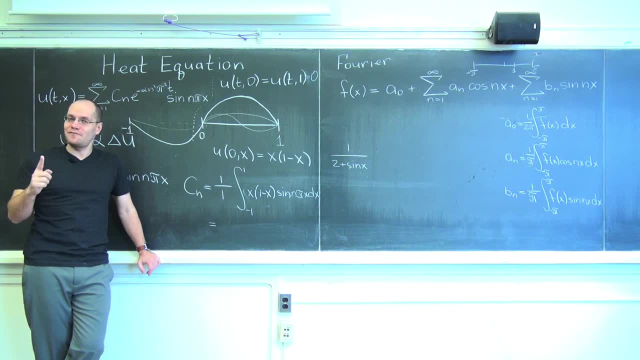 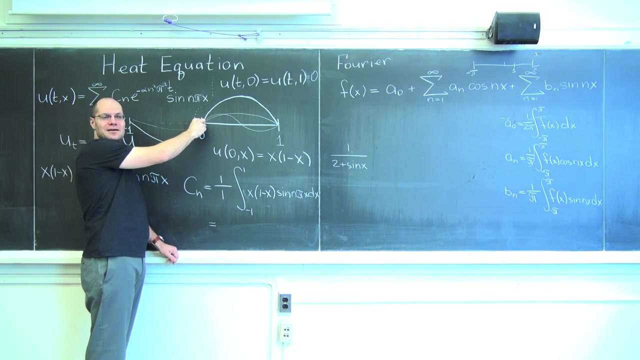 so hold on, I'll tell you what I think if it's continuous. so here's what fooled us. I'm putting myself in that category because I was fooled also, like this looks perfectly smooth, but it's definitely not, because if you think about the second derivative, if you go to the second derivative, 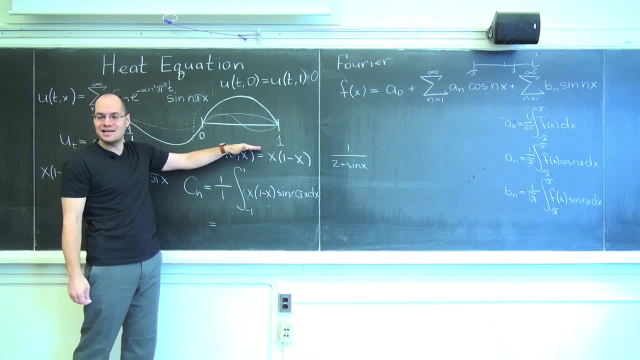 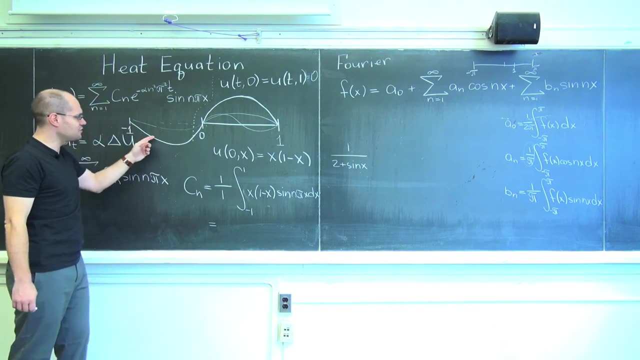 this is a parabola and this is a parabola. so for this derivative it will be a negative constant and for this, excuse me, for this part of the parabola, it will be a negative constant and for this part of the parabola it will be a positive constant. 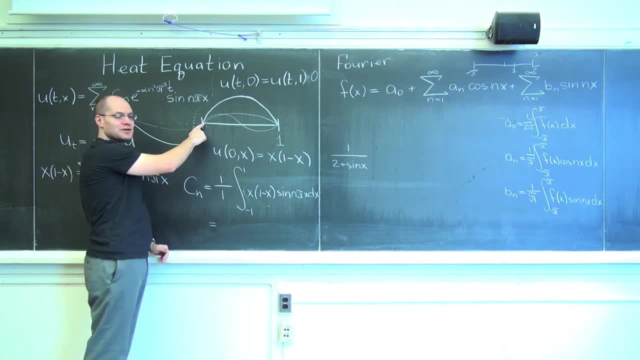 so obviously there will be a mismatch here. so this point is not as smooth as it looks in chalk. it's a little bit of an optical illusion. it's definitely there's definitely there something discontinuous there, but I only think it occurs in the second derivative. 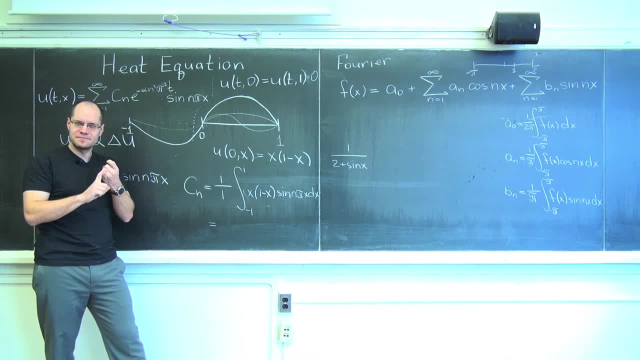 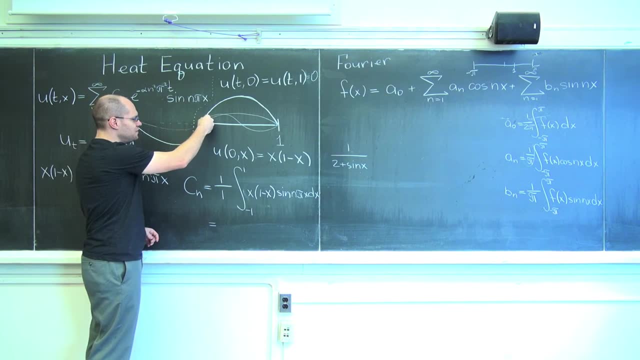 so I think that the first derivative, the function itself, is continuous, and I believe its first derivative is continuous as well, just because when you reflect something, whatever the tangent is, it just stays there and becomes itself. when you reflect something in the rotation, by 180 degree sense, 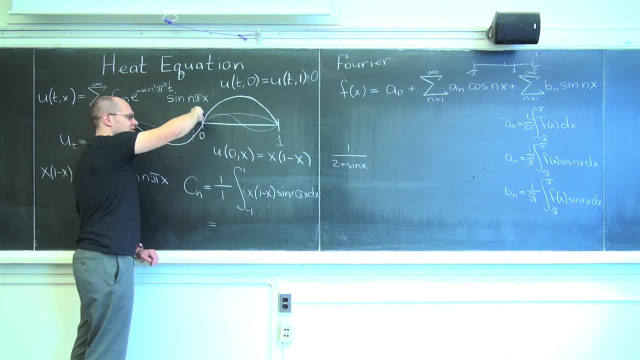 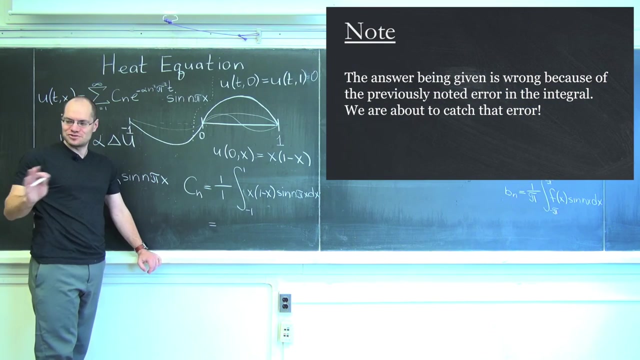 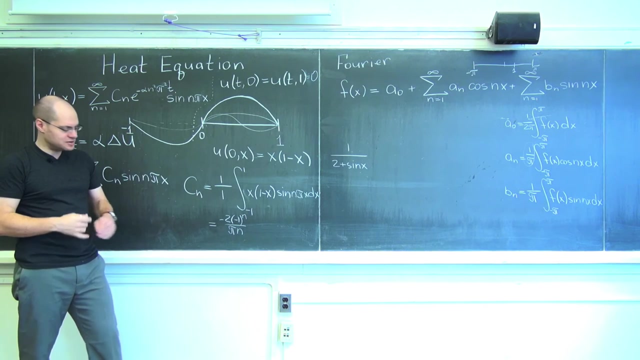 it's basically reflection with respect to a point. so the tangent flips 180 degrees and becomes itself. so I say they decay as 1 over n cubed. was I right? no see, I don't believe that, because that would mean that the function is discontinuous. 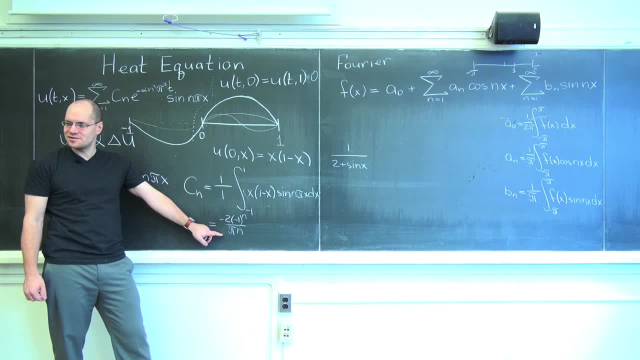 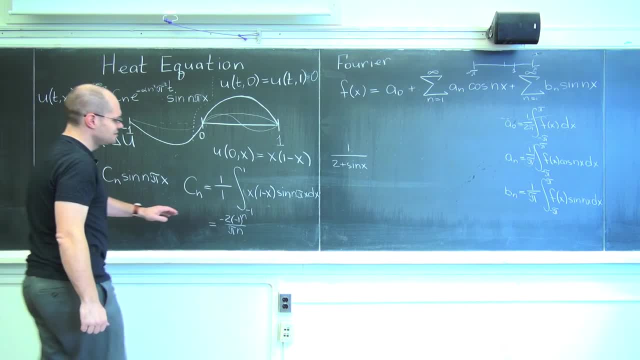 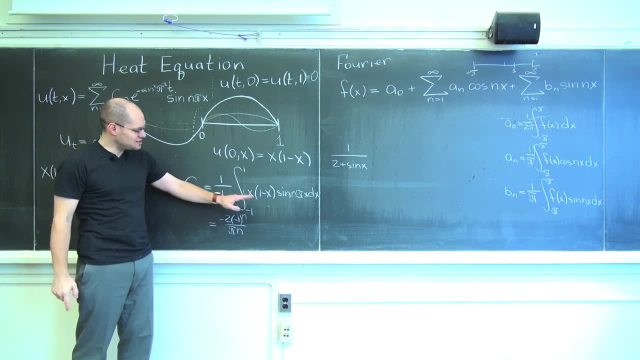 no, okay, okay, I'm sorry. yes, okay, my fault. I take full responsibility. so it's not this integral, that's the mistake, because this function on the left is not, is not x times 1 minus x, it is its flipped version. it is a different function. so 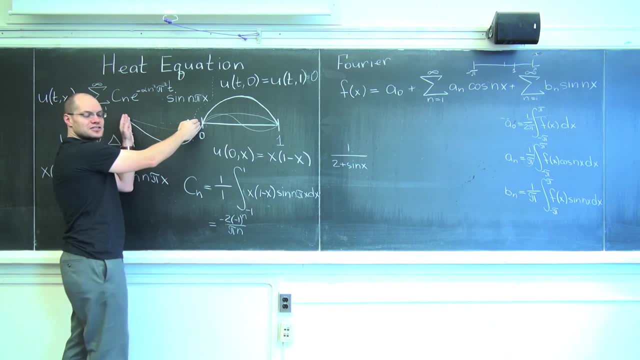 what we should have really done. so it's this integral plus a different integral here. the function here is x times 1 plus x. that's what this is. this is x times 1 minus x, but when we reflected it the way that we did, this portion of it. 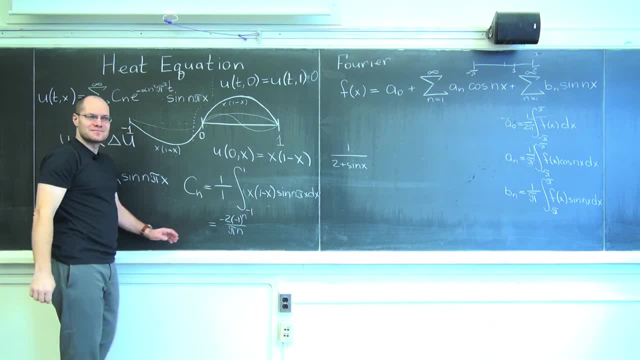 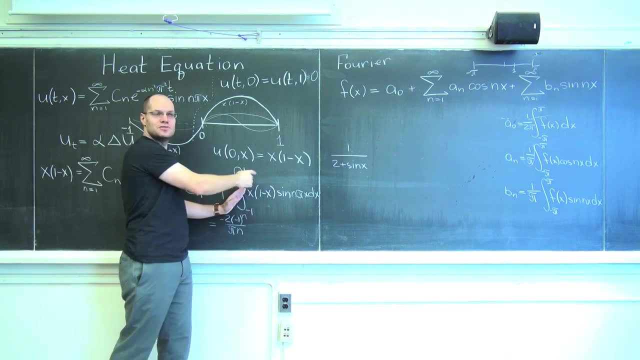 is x times 1 plus x. so what we should have done is we should have made this from minus 1 to 0 and this from 0 to 1, and, of course, what it will become is twice. where do I put the 2? twice this integral? 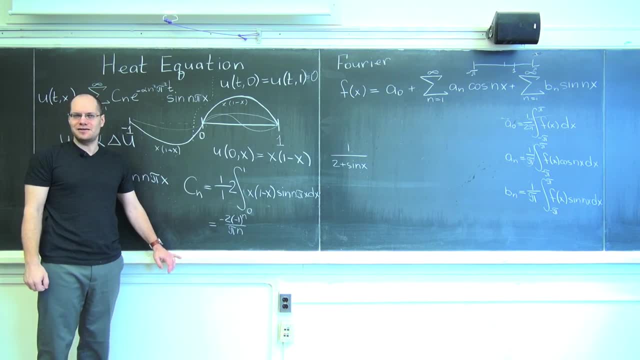 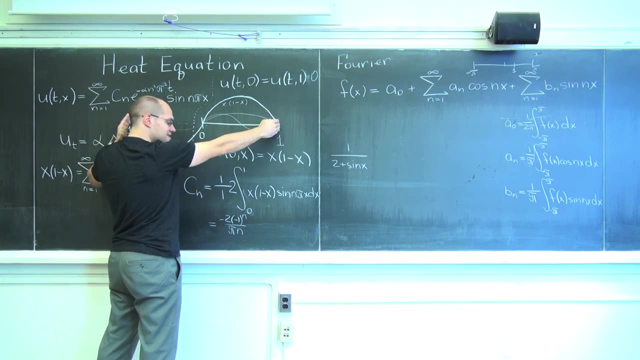 from 0 to 1. are you guys with me now? do you see the mistake that we've made? no, because we're now going after this integral. this is the integral that we need, with something here and something slightly different here, and that combined integral is whatever we had here. 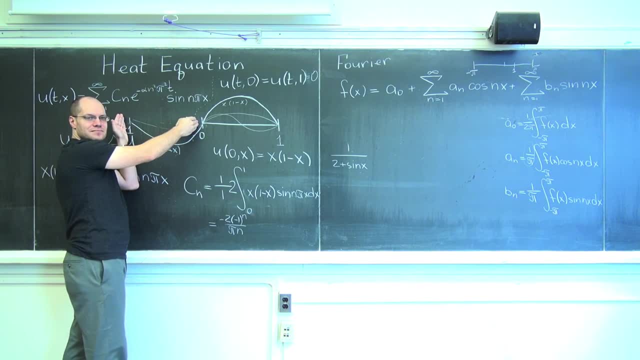 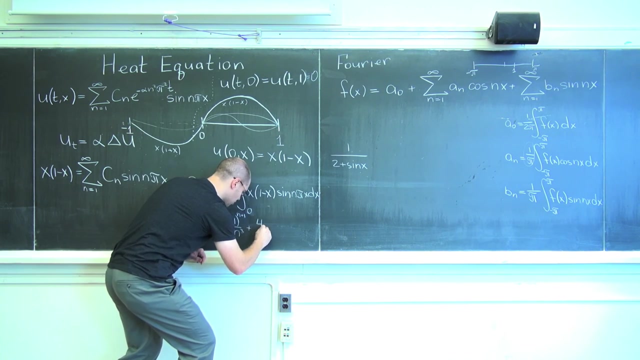 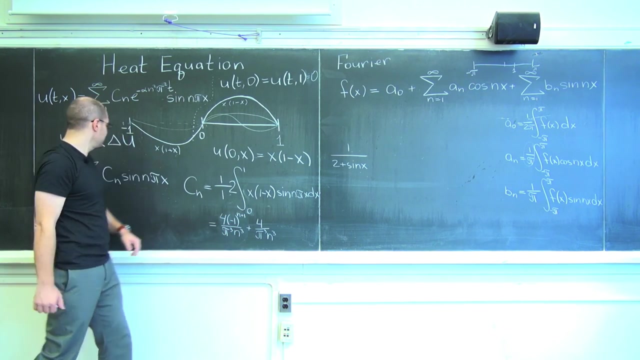 times 2, because whatever we have here is the same thing. yeah, so this is your new integral, so from 0 to 1 and then multiplied by 2, so I think we can definitely combine them: 1 plus this. okay, so we have solved the problem. 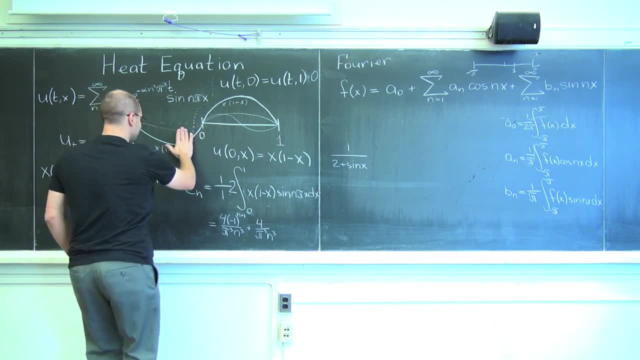 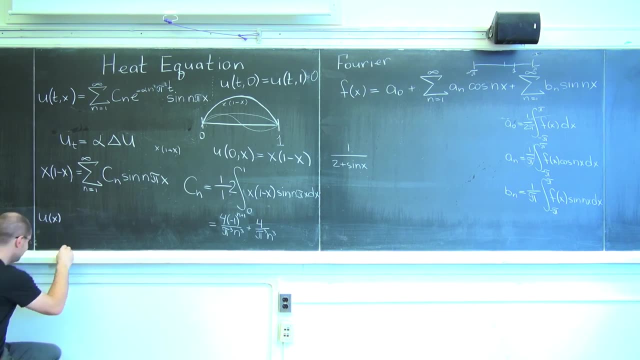 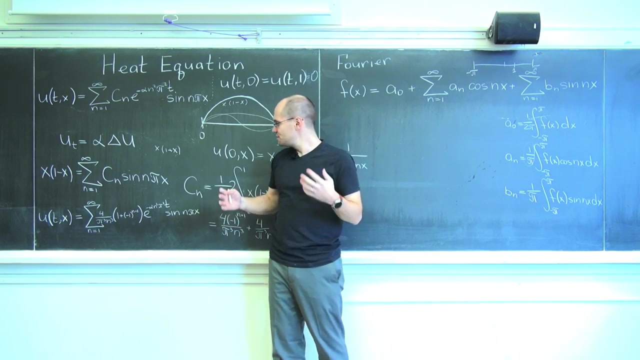 and we can now just actually write down its solution. let me erase this and I would say that this is our first non-trivial PDE and it was solved from start to finish.